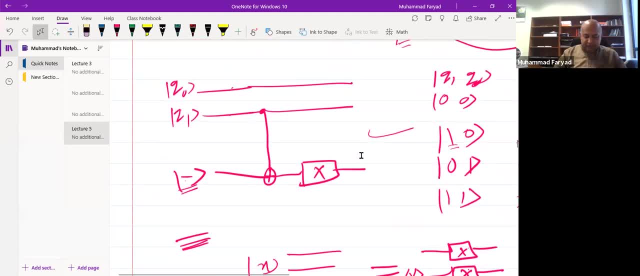 these phase oracles, using essentially circuits of this type, that we have several qubits and then there is an auxiliary qubit which is set in this minus state And different. you know, balanced function essentially means applying different combinations of these C and that's it. 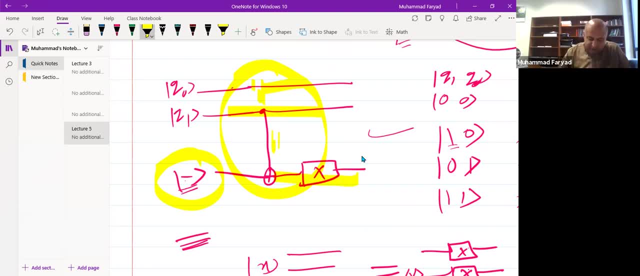 You know, if you change the location of C, for example from here to here, and you implement another C, All you do it is still a balanced function. The only difference will happen that these four combinations for which you get a minus sign, they change Like if the one. 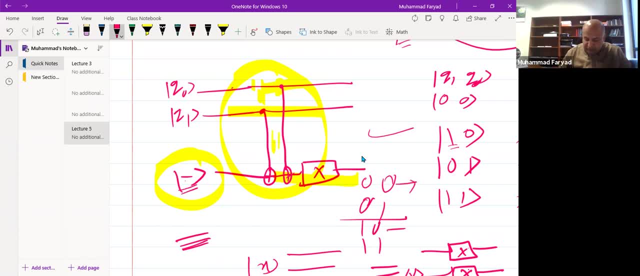 gave you, f is equal to 1 for this and this, adding another one, might give you one for you know, for this or this input and so on. So we can also have you know an x gates before this CK, creating a vo not gate, and that can you know. change again these x's, for which the output would be one. 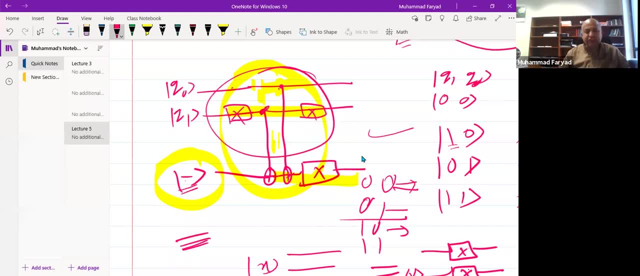 But all of these implementations will still keep. it will still make it a balanced function, Because half of the input will map to 1 and the other half of it will map to 2, because that's all so. thankfully, it's very easy to teach it. Let's go on with the'rex gates. ζ. 1, assert the length. We know that in time is enough to know how to always observe complex relationships. so first you know that Java should have single and equal assertions along the lines, while you set so many operations with bad tych frames. because 401 is not walkthrough is also moving. 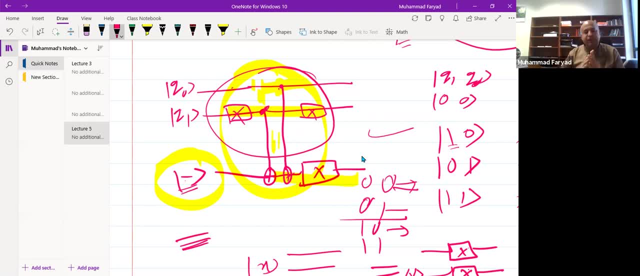 So as kinds of native x gates, where you call it, these吃obyった現在 you should- input will map to one and the other half will map to zero. So we will implement balanced oracles using this function. So this X is not needed, as we will work with this keeping. 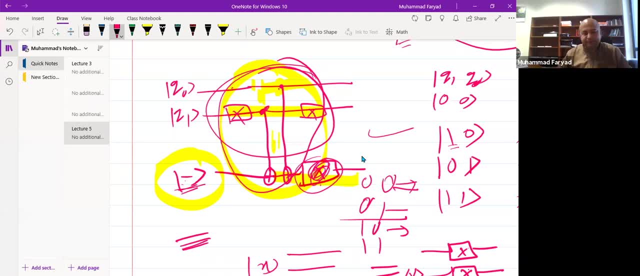 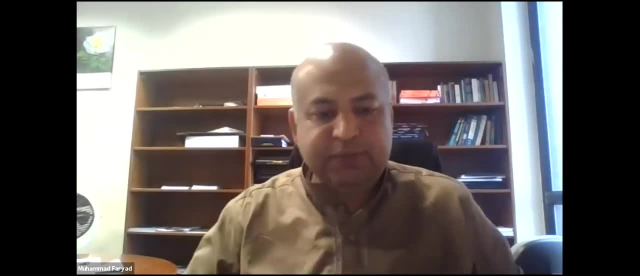 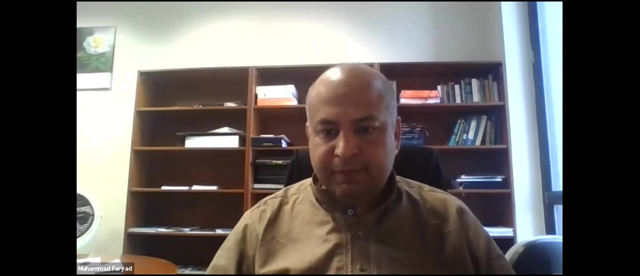 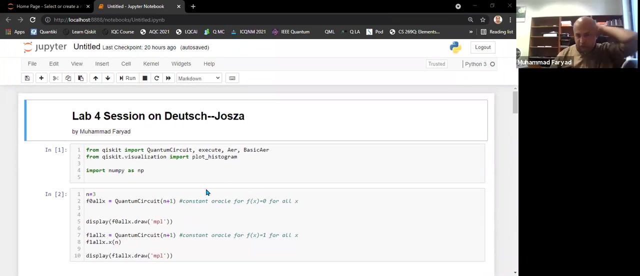 in minus one and nothing doing to it except for control X. Okay, so let me unshare this thing and share my screen. So start implementing this function. Okay, So there are two ways for me to show the implementation of the circuit. One is that I walk you through the program that I have already written. 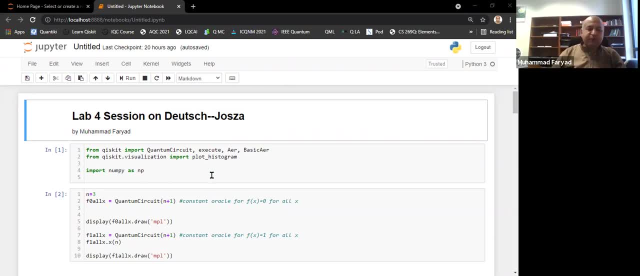 and the other one is where I write the program myself. I wrote the program, you know, myself in the last couple of sessions, But from now on, you know, I can prefer walking you through the program that I have already written and sharing the notebook with you. 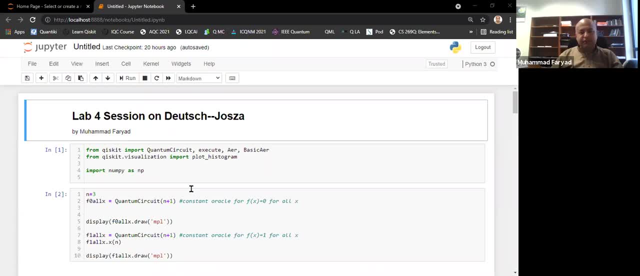 But if you, you know, feel like that you will get better if I keep typing in front of you, then please do let me know. Okay, So let me Let me see if I should increase the size of this thing, Okay, 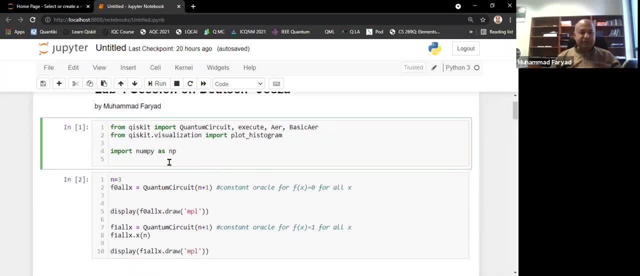 So I will increase the size a little bit so that you can read it easily. So this first you know box input box has just usual imports. I'm importing a quantum circuit, execute air, basic air and plot histogram. 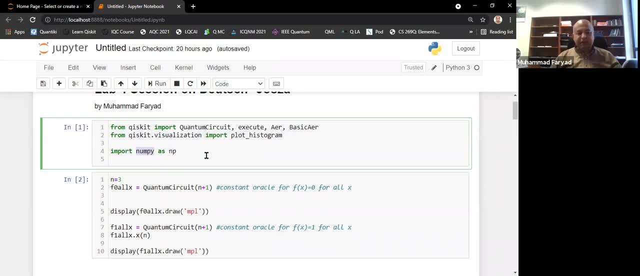 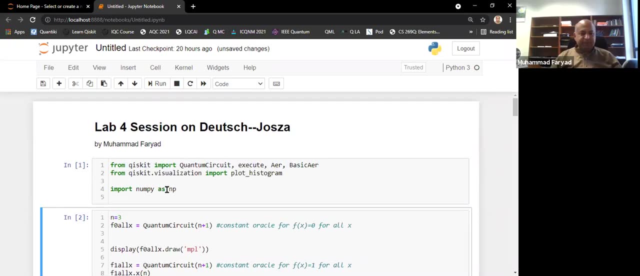 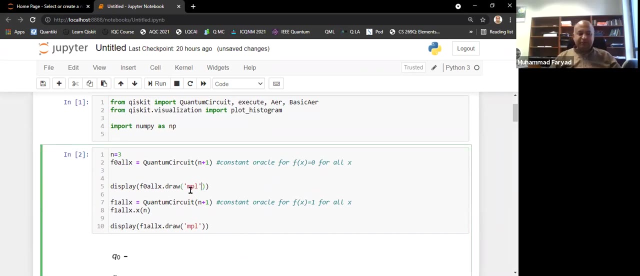 And of course we need Numpy many times. So let me shift, enter this, Enter this one. So this is a star, so it's still running. Now, here I have constructed two constant oracles. So this first oracle, I'm calling it F0, all X. 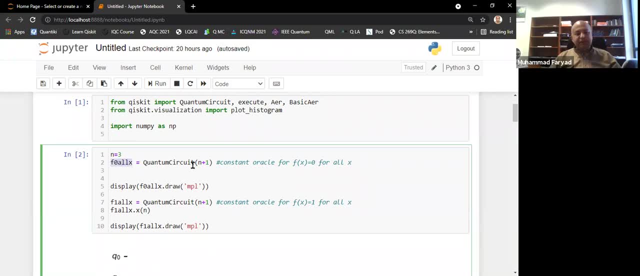 Okay, This means that this will implement, you know, a function: F is equal to zero for all X. So what type of oracle this should be? This should be an oracle, Okay. So the way this works is that whatever the input is, the same goes at the 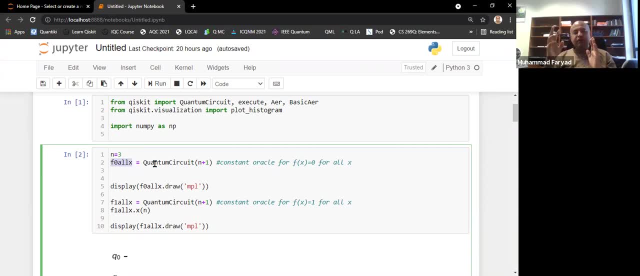 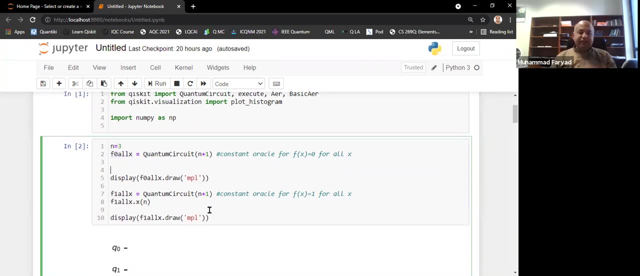 output because F is zero. So if f of X is zero minus one, raised to power, zero is one. So no phase is being added to the input. So essentially that is all that there is. So let me take this thing out and run this. 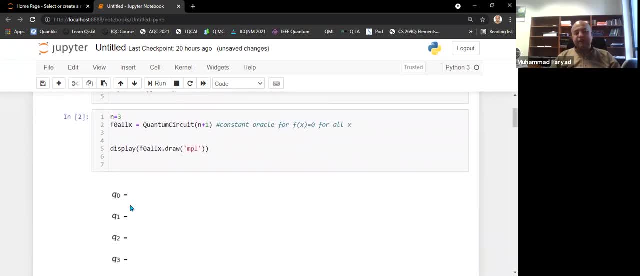 And you see, this oracle is nothing but just four qubit as it is, because whatever is at the input, the same, okay, so everybody's okay with the. this oracle for f of x is equal to zero. perfect, all right. so let me add another cell at the bottom and 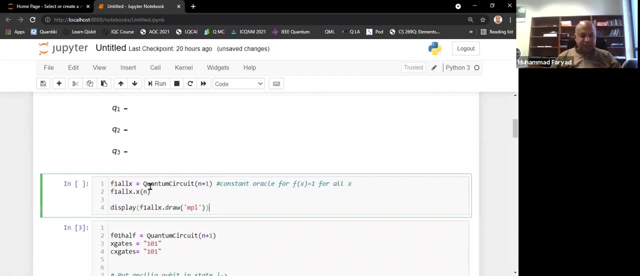 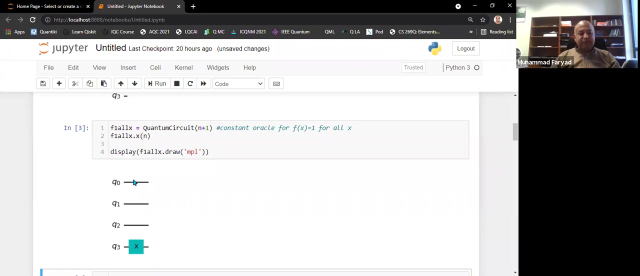 uh, paste the other part here. so this is an oracle that i have created, for f of x is equal to one, which mean that since f of x is one for all x, so for all inputs, i should get a minus at the output. so let's see what there is. and now you see that instead of inverting my three working qubits q0. 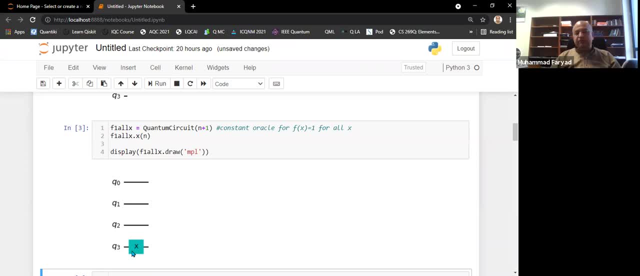 q1: 2. i have inverted the auxiliary uh the, the ancillary qubit, and the reason is the same as i uh discuss in at the end of last slide, that uh, in quantum mechanics, the global phase uh which appears, you know, uh, in front of two product. 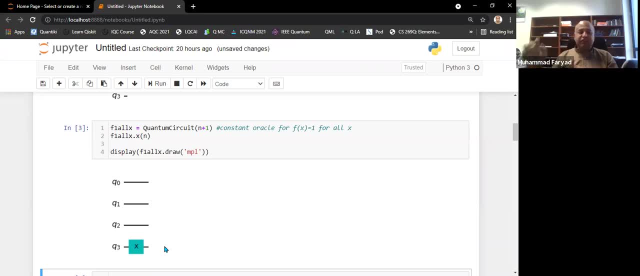 states can be thought of with any of the you know state. so if you think of this q0, q1, q2 as one state and this q3 as the other state, this x is going to add a minus sign if this q3 is in the minus state. 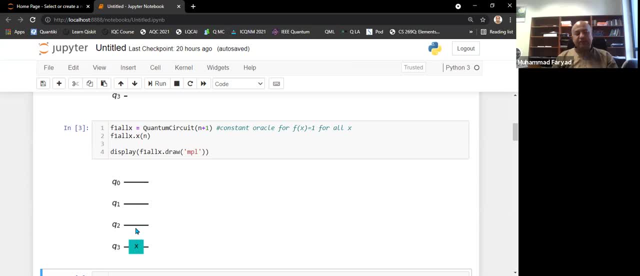 so it doesn't matter if you put these three in x and don't do anything to q3, or if you put x here and don't do anything to q0, q1, q2. so in so if we put x in front of these three, it would be, you know. 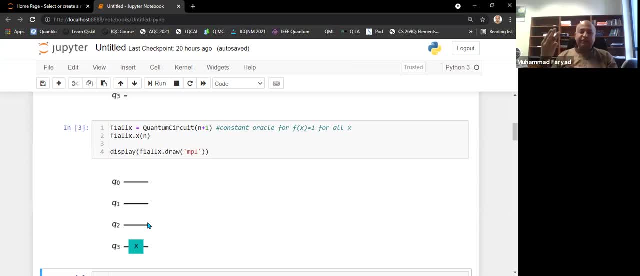 a little bit of overdoing. we will have to execute three x's instead of just one x, so that's why it's preferable to implement f of x is equal to one oracle, uh, with an x on the ancillary qubit instead of x on the working qubits. so is this okay? 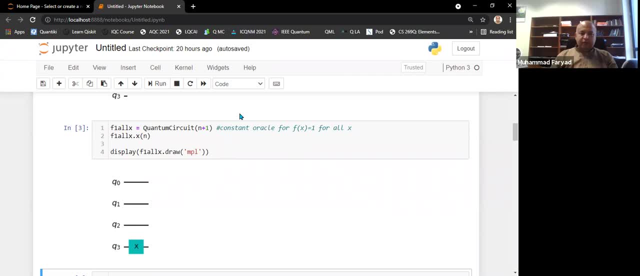 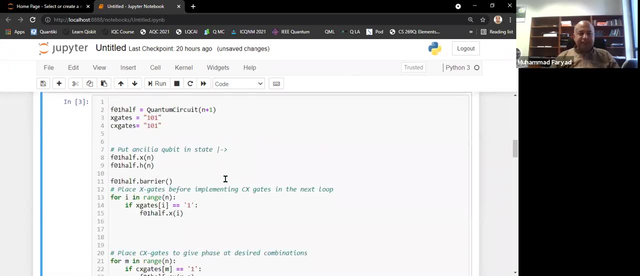 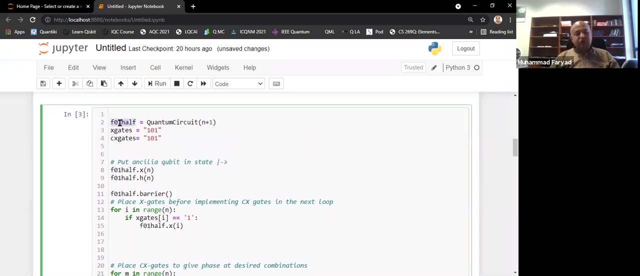 all right, so let me go to the next part now. now, this is a part where i construct uh, an oracle, which is zero for uh half of the input and one for the other half of the input. so let me just write a comment that this implements: an f of x is equal to zero, or half of inputs, and f of x is equal to one. 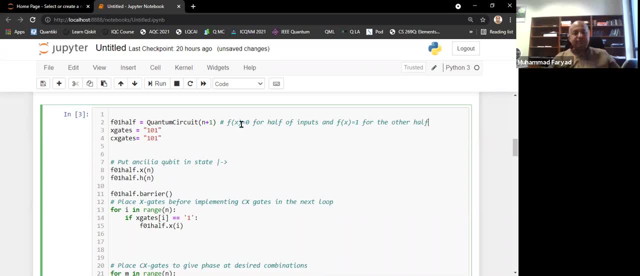 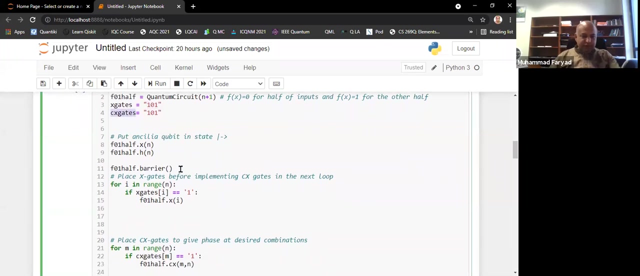 of the other half. now i have prepared two strings, so this is a string 1 0, 1. and then this is i have, i'm calling it x, k string, and you will just see- uh, you know the reason for this shortly- and then i have a cx gate string, which is again 101 for the moment, and let me you know, take this part. 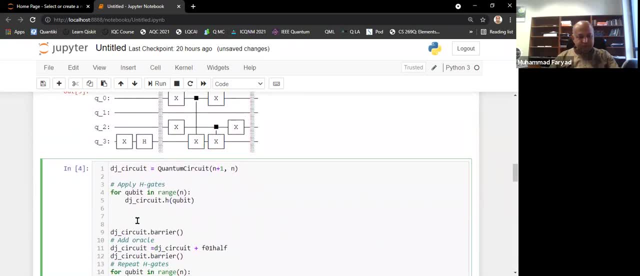 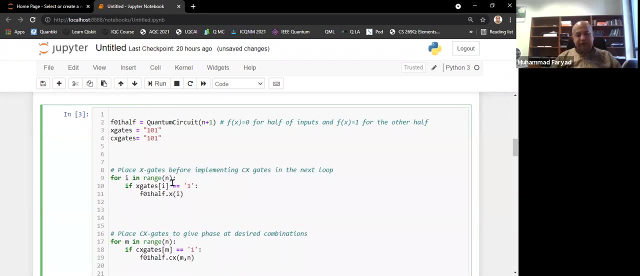 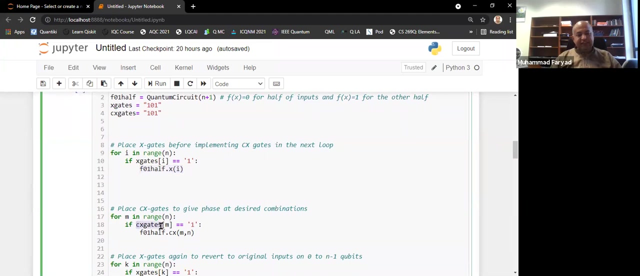 to a part in the next part for now. so now i have after this. is that what i do, that i implement this loop far over these x gates, this string, and i say that whenever this x gate term is 1, what you do, you implement an x gate. and for the cx gates i do the same. i run a loop over. 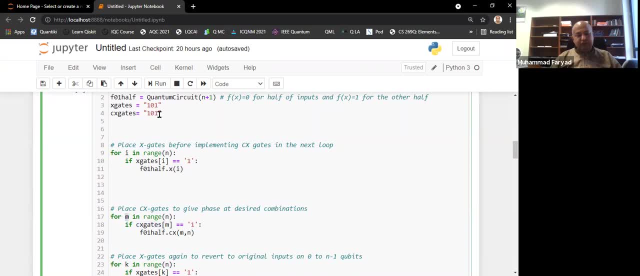 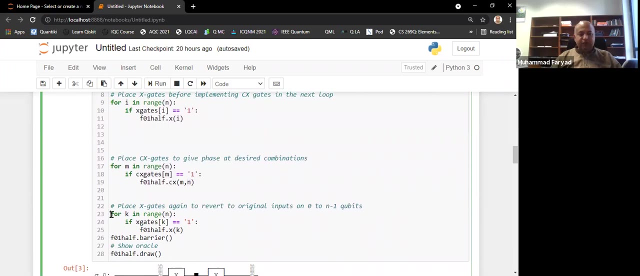 this cx gate. you know string and i say that whenever it is one, implement a cx which is being controlled by a string m, but all cx are being implemented on the nth qubit, which is the ancillary qubit, and then at the end i have to apply x gates again, just because i want the same input. 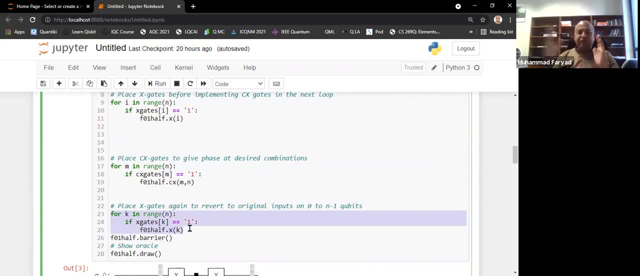 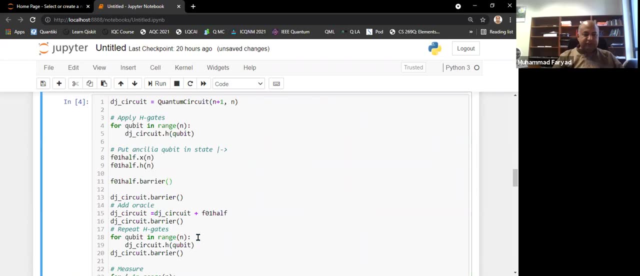 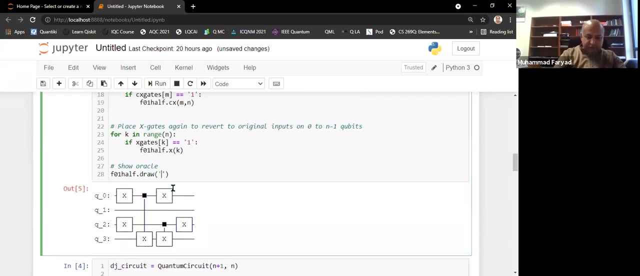 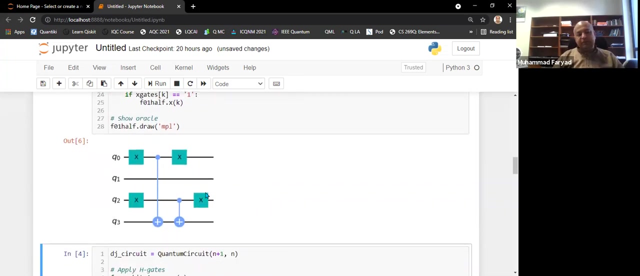 same output as the input on the three working qubits and let's say i have a barrier here. but let's remove this barrier, so let's run this. this is a circle. let me draw it. mpl. now, you see, this is my oracle and, as you can see, that this implements some combination. i'm not 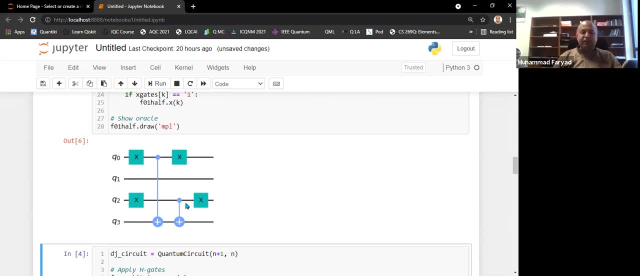 worried about for that right now. but this is a balanced particle because it's implementing these control x gates and you see that for all of these control x gates, i have a barrier, which is the one that is running on the nth qubit, which is the input on the three. 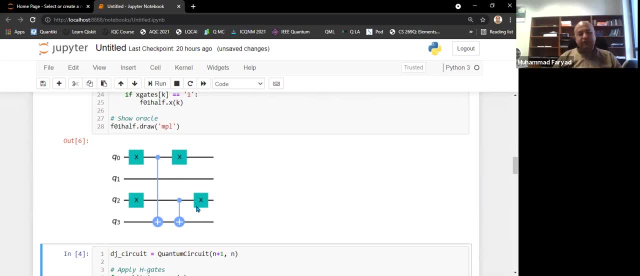 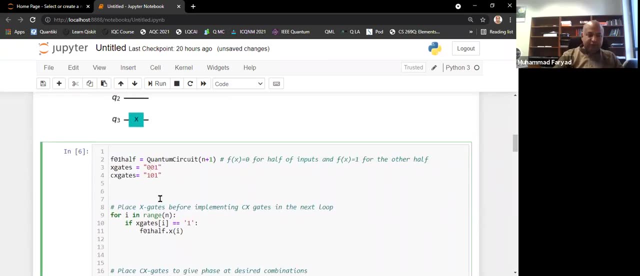 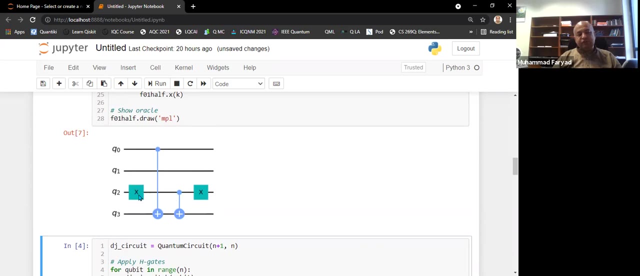 i'm putting an x gate before and after. just you know to get different combination what you can do. you can also have, let's say, some c control x without any x before and after, and some control x with some, you know, x before and after. that's how you can have various combination here and the number where you 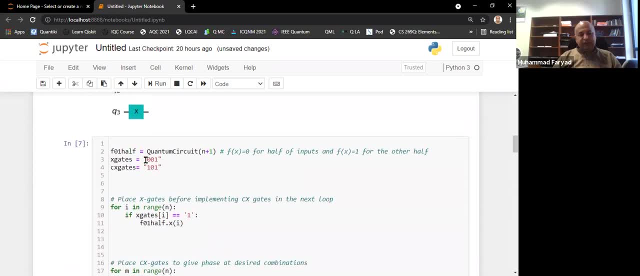 want to put the cx gate. you can choose this with string. i mean, these are only three qubit. if you want, you can do it without any loops as well. you can just, you know, and code directly: okay, apply this cx on these two qubits and this cx over here and this x over there, etc. but you know, this is a little. 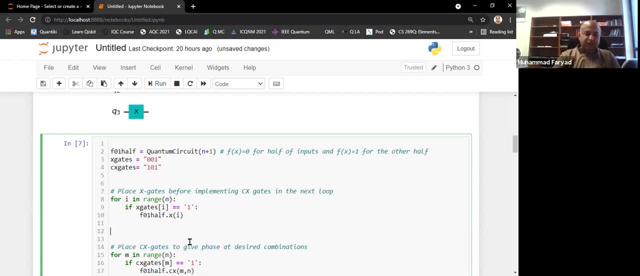 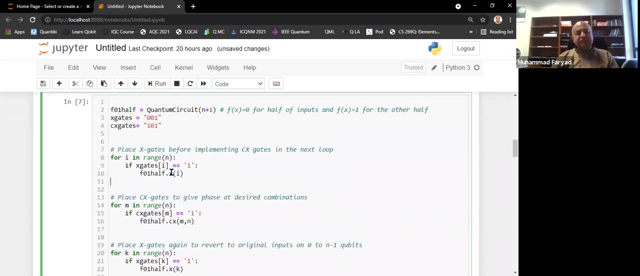 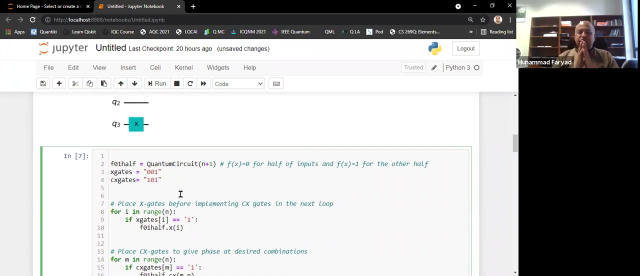 bit a nicer way and also scalable very easily, because if you have to make a circuit for 10 qubits, you know it's much easier to define these strings for x gates and control x gates and then say, okay, you, you need a control x gate at this, this place and and an x gate at this, this place. 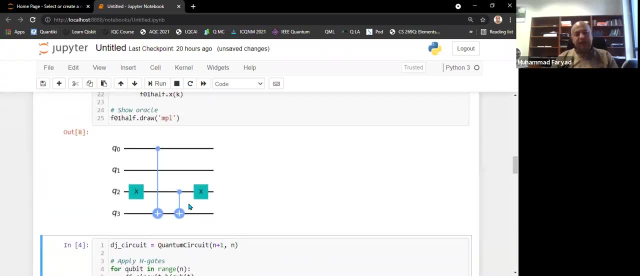 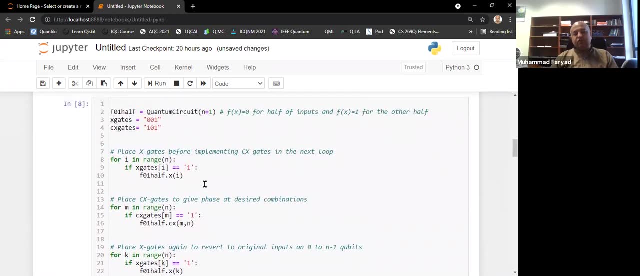 and this can give you a balanced oracle like this. we have an activity where you're supposed to make a balanced oracle that you know transforms minus with minus sign for particular inputs and other four with a plus sign. so then you will have to think what combination of x and 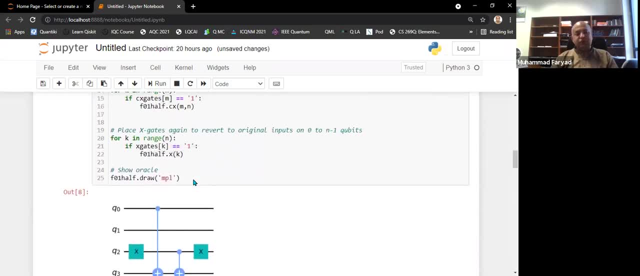 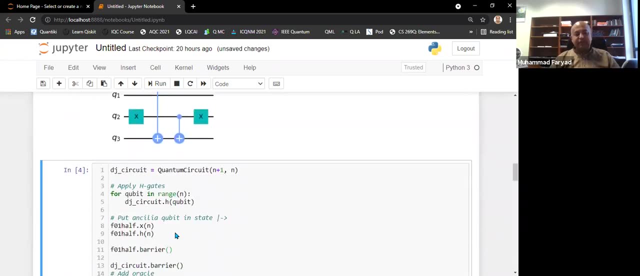 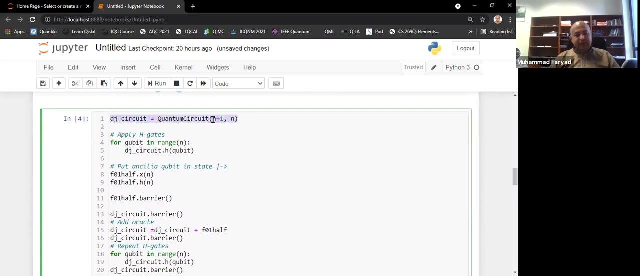 cx gates you have to use, but for now i'm just, you know, giving it as a general one, so you can take any one, okay, so this is a balanced oracle and let's now go to the dice. josa circuit. so this is a circuit, again, that have n plus four. 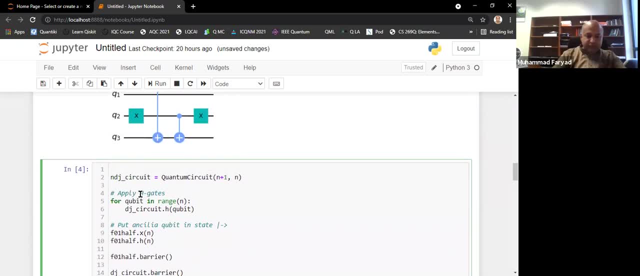 one quantum bits. and let's say i put n is equal to three here again. so it has four qubits and it has three classical bits. so in a quantum circuit i can specify the number of classical bits and number of qubit. by the way, if you just 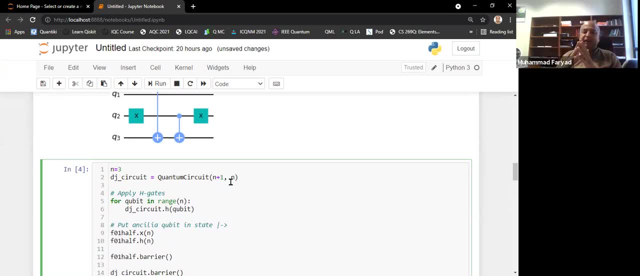 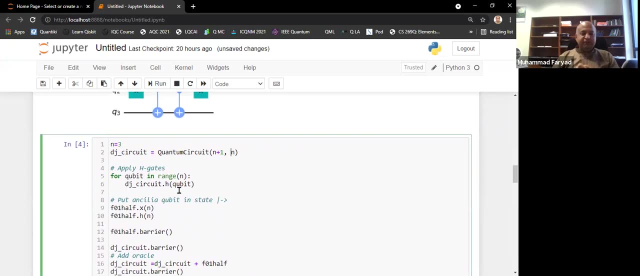 give only one input, then by default it will consider them as qubits, not not classical bits. all right, so this circuit is actually really, really simple. uh, what you have is a loop that i have this variable qubit, you can have it, i jk doesn't matter, but qubit, you know, as a variable. 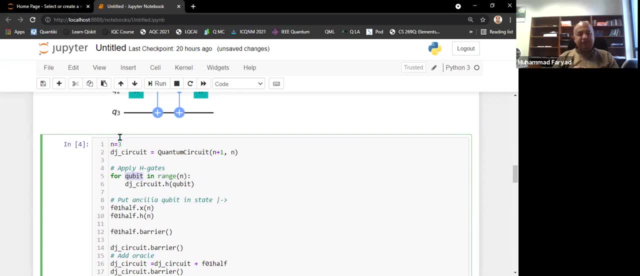 looks a bit nicer. so in the range n is three, qubit will go from zero, one and two. so in python it starts, index, starts at zero, and when we say this range it goes to n minus one. so this is three. so it will go to two. so zero, one, two. so 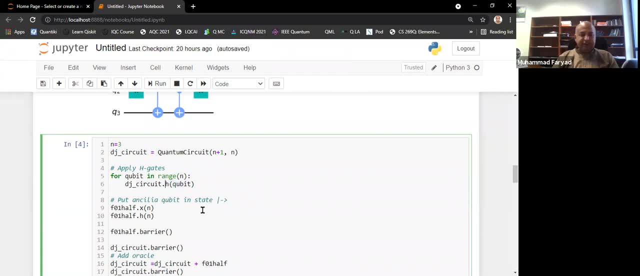 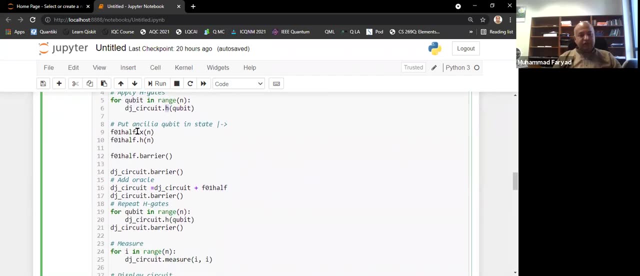 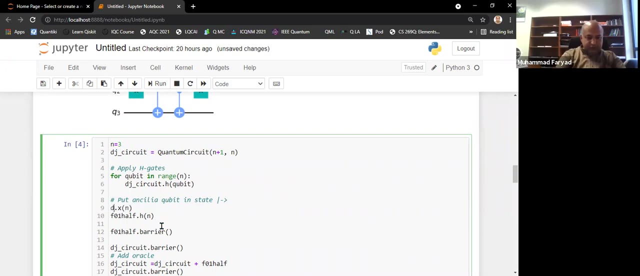 at these ql locations, i'm applying a hadamard gate, you can see here. so i have this series of adamant gates and then, uh, you know, this is the part with. just let me make here, this is the day circuit, and you can see that these two commands simply put: uh, this, uh, nth, qubit in in the minus state. 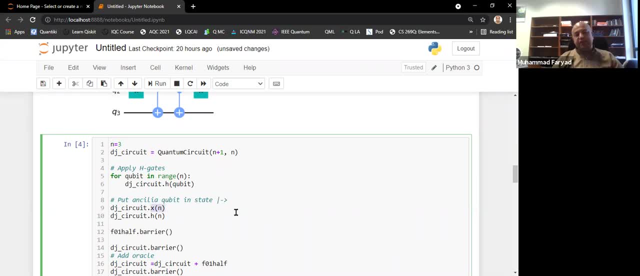 because first i do this x gate x, because by default each qubit starts in zero state in python. so this x makes it one. and then this hadamard h, it makes it minus state because one goes to minus under hadamard. so this you know. 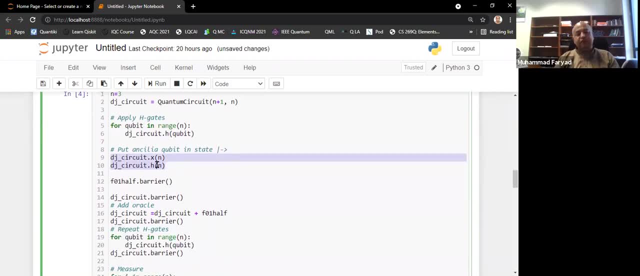 uh, transform my last qubit, which i will use as an insular qubit, into the minus state, and then i let me add this barrier for visualization help, okay, so let's move this all right now. you see, this is a nice way of adding oracle right here. 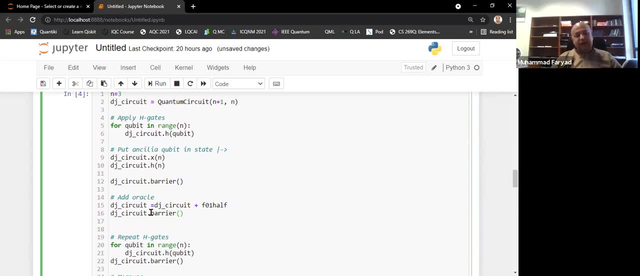 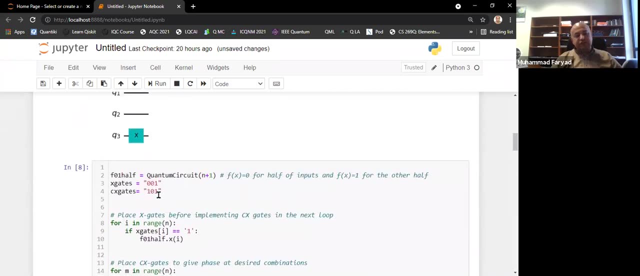 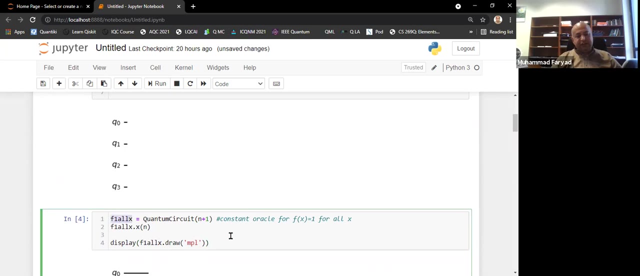 and all i'm doing just specifying which circuit that i have already defined here. you see, i have given names to different circuits. so this is f zero one half. so this is my balance circuit. this uh f one all x is my one constant function and f zero all x is my other constant uh function. 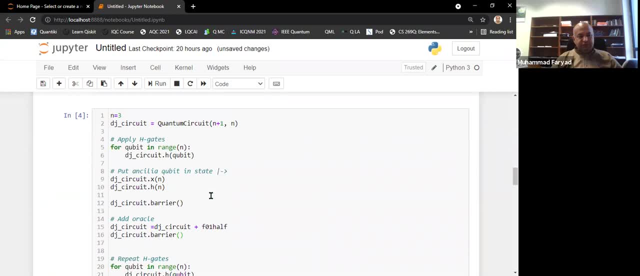 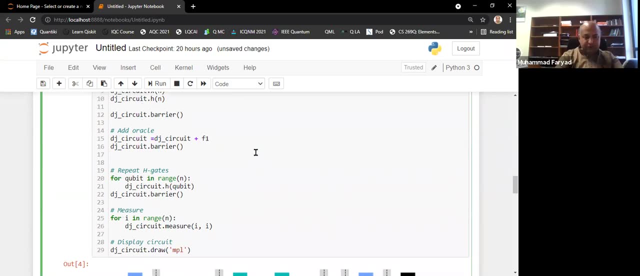 so over here i can choose uh, uh, whichever i want. so let's say, first choose f1, all x, and then i just put this barrier for visualization purpose. now, once i have introduced this uh oracle in my circuit, in this dj circuit, i'm putting these uh hadamard transforms again. so this is just the repetition. 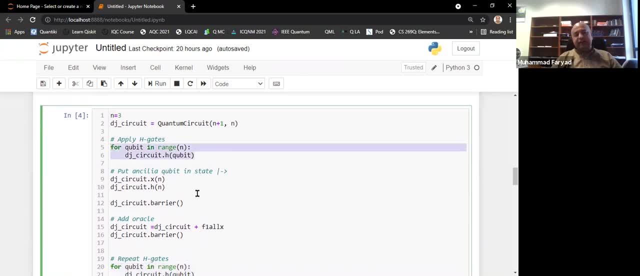 of the same uh loop that i had over here again, this is a three qubit circuit. you don't really have to use loops, you can, uh, you know, in three lines just specify hadamard and zero, head about one, had another two and that's it. 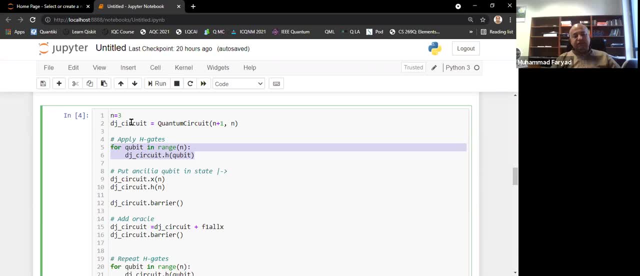 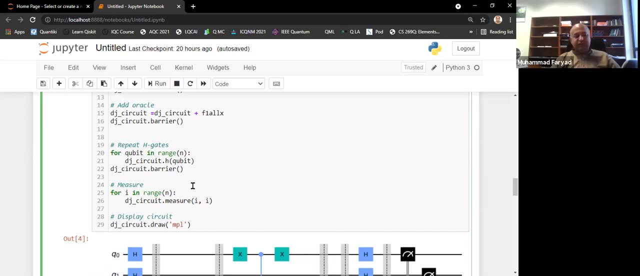 but you know, this is a little bit scalable, that later on if you need to increase this end, you can just you know, uh, this will automatically scale to the naughty value of n. okay, and then at the end i add these measurements and you see, for a measurement i need to specify. 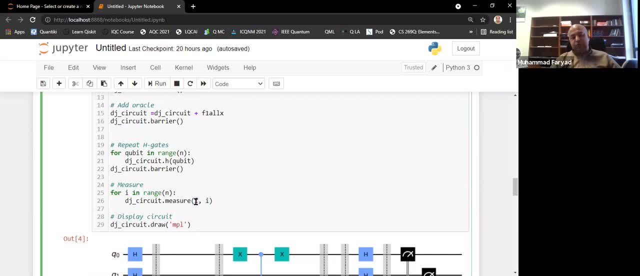 the qubits and the classical bit that i measure ith qubit, where i is going from zero to one n minus one, because this is range n. so when i give range n in python is it goes from zero to n minus one. so my zero to n minus one qubits are being measured and their results are being 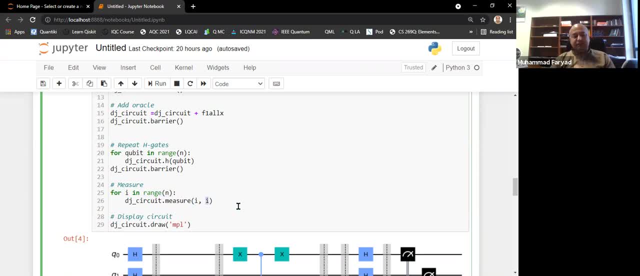 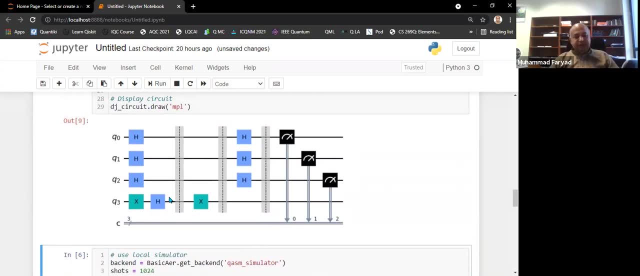 copied to the classical bit corresponding classical bit. so let's run this circuit. so here is the circuit, and you see that this is the hadamard transform part. this is the part where my qubit and cilia is going from zero to minus. and this is my constant oracle right now, because 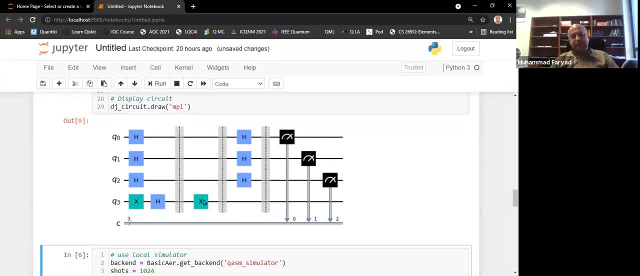 with f of x one. so i'm just flipping this one, which is equivalent to flipping these three, and then i have these hadamard, and then these measurements, these barriers are just for purpose and doing nothing. all right, so let me stop here and ask if there is any question. 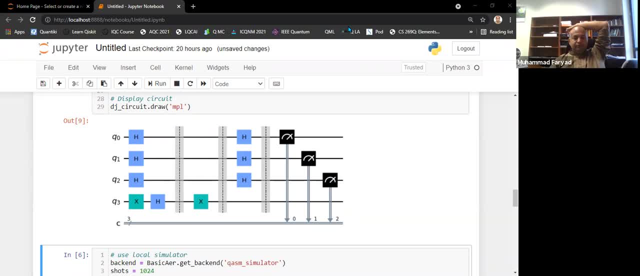 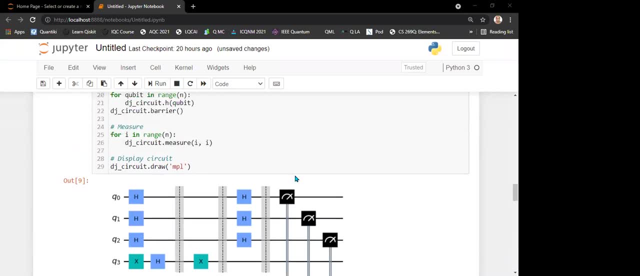 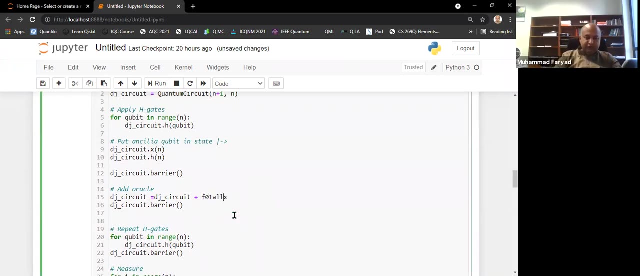 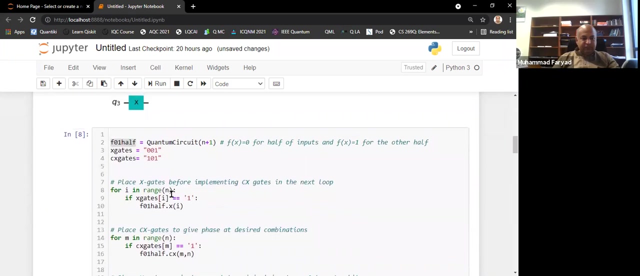 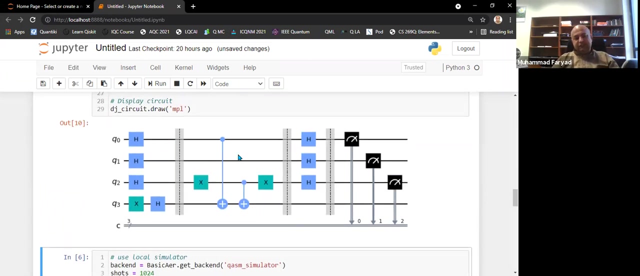 no, all right. so let me just show you, for example, i add an f zero one oracle here, which i have given a name f zero one half. let me check: yes, absolutely one half. so if i use this, then this is my circuit. okay, this part here between these two barriers, is the ballast oracle. 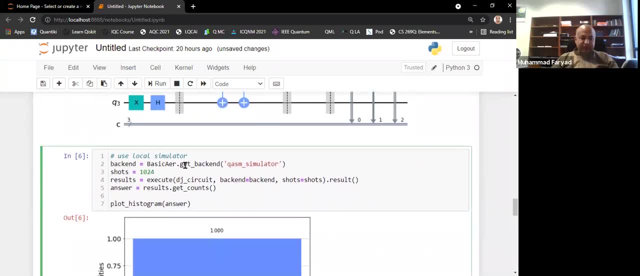 anyway. so let's now simulate it, and for simulation i'm using the same structure as before i have. i'm going to first use this cosp simulator, which is the simulator provided by ibm, and then i'm specifying number of shots as 1024. there's no reason to have you know, it has a 1024. you can have it as 1000, but since a lot of people 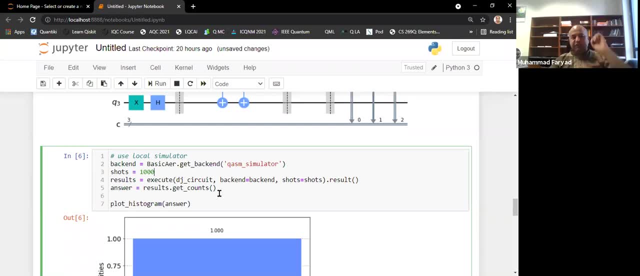 are coming to this quantum computer programming from computer science background. so some people, you know, prefer to go in power of two. but you know you can specify these number of shots to, you know, any value you want. okay, and then i have this job that i'm calling this results. so this results. 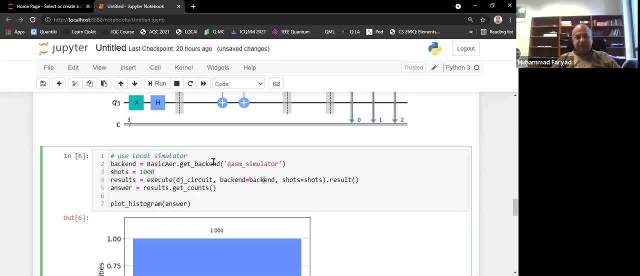 uh will execute this dj circuit with the back end, that is, uh provide over here with shots equal to 1000 and i'm collecting the result from this and putting it. results variable and from results i'm getting uh counts, we, we can get other things from results as well, which i will. uh, uh, you know. 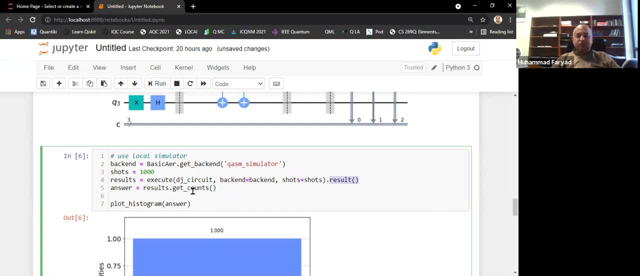 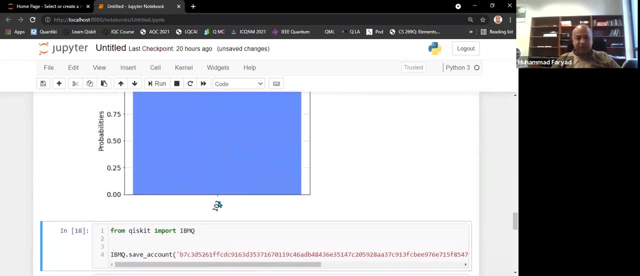 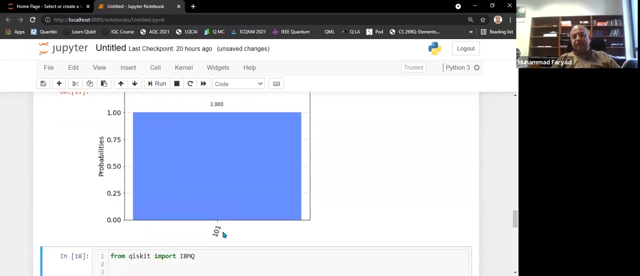 also do in due course, but right now we are just interested in counts and then i'm plotting it using histogram, so let's see what output we get. okay, so we got 101 state at the output with 100 probability. so this means what? this means that the uh oracle that was implemented. 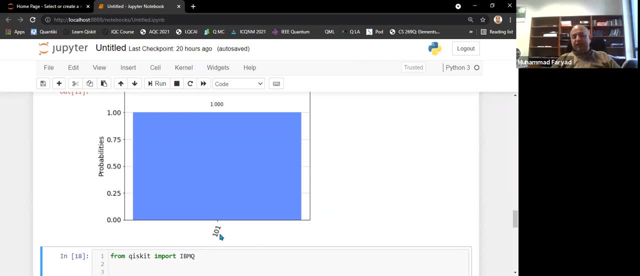 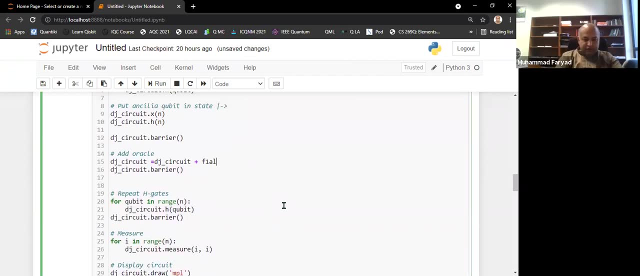 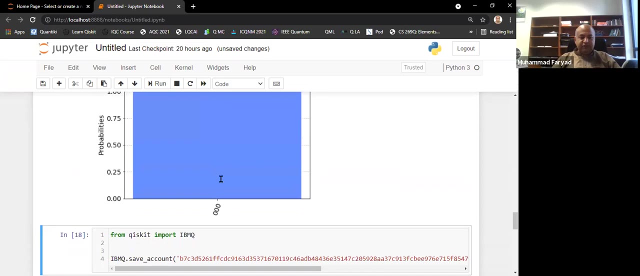 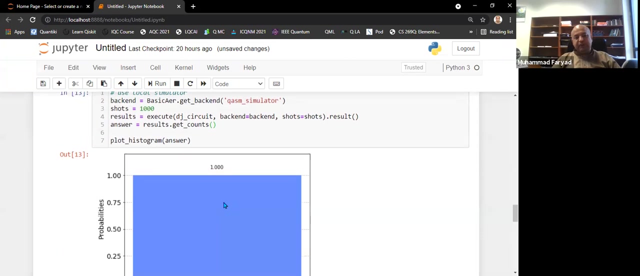 uh was a balanced oracle, because i'm getting something other than zero if i had specified here, let's say, f one for all, x, this one. so. so now i have a constant oracle. let's see. so you can see, my output state is zero, zero, zero. so this zero, zero, zero state is coming with 100 percent probability. so which mean that 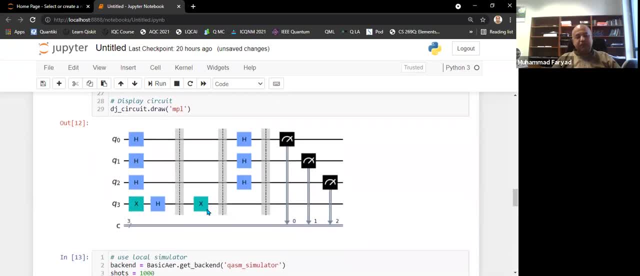 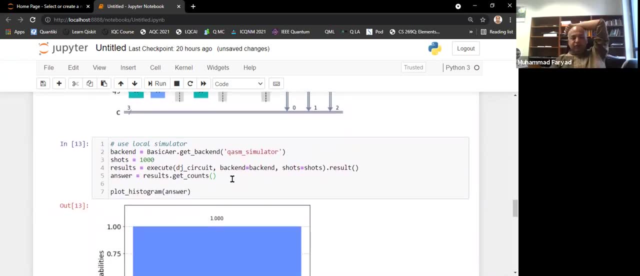 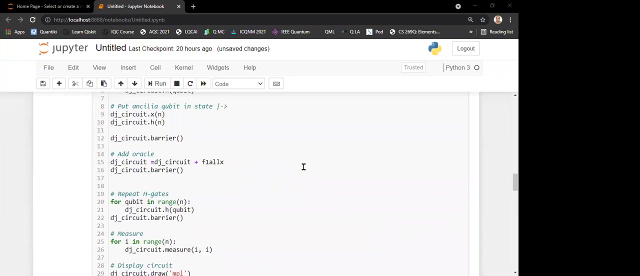 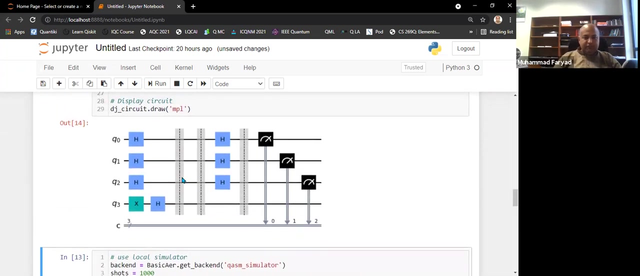 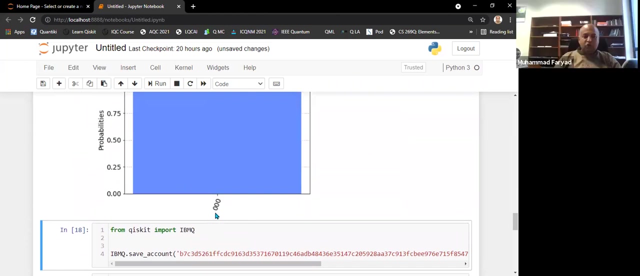 my computer has found that my oracle is a constant oracle, so any question, so far perfect. so by the law, you have raised uh hand, please go ahead. i'm yes, so for f, zero, all x. so i have this circuit with the nothing happening, these input qubits, and again my output state is zero. zero with the 100 probability. 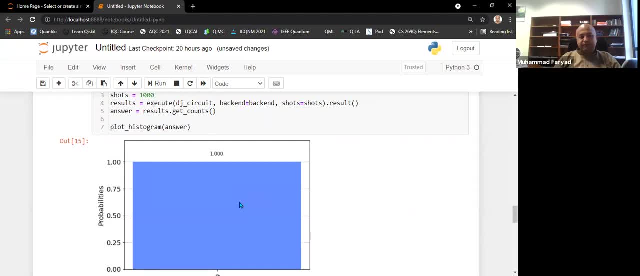 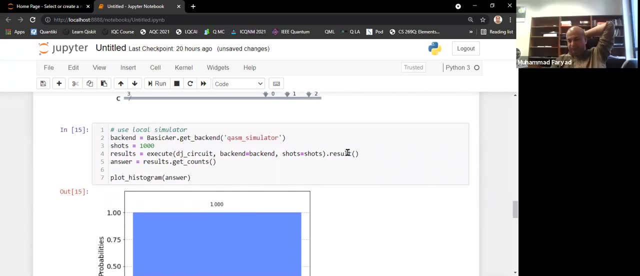 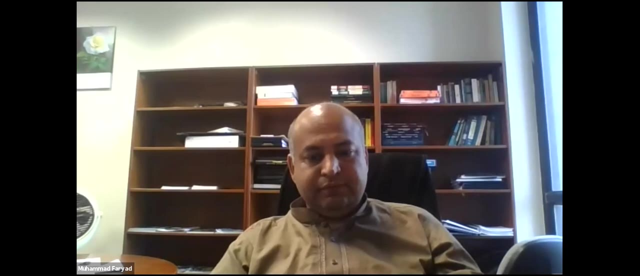 so it means that my oracle is a constant oracle? okay, thank you. perfect, so any other question? 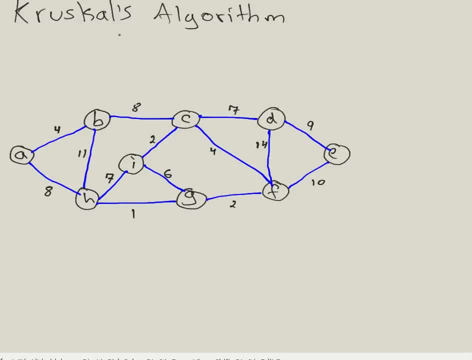 Alright, so today I want to talk about cross-course algorithm, which is easy and pretty straightforward. The basic idea is to select the least costly edge UV and keep selecting all the edges that are least costly until you reach all the vertices in your resulting minimum spanning tree. 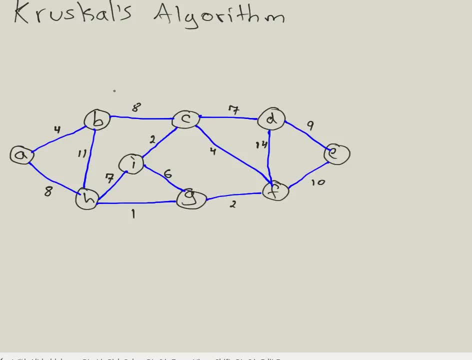 The only thing is you can't have any cycles. But everything will become clear once I work through this example here. By the way, this graph is taken from the Corman's book. So let's begin. So you start with the least costly edge. 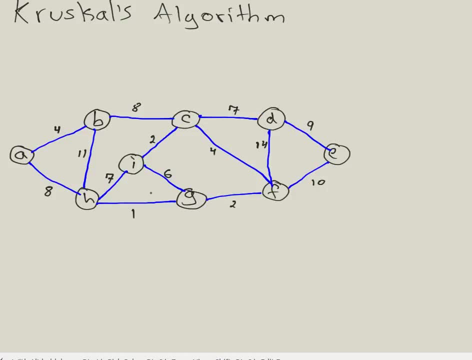 By the way, if you had another one, like if there was another edge with the cost of 1,, it wouldn't matter which one you picked as your starting point. In this case, there's only one edge with cost of 1.. 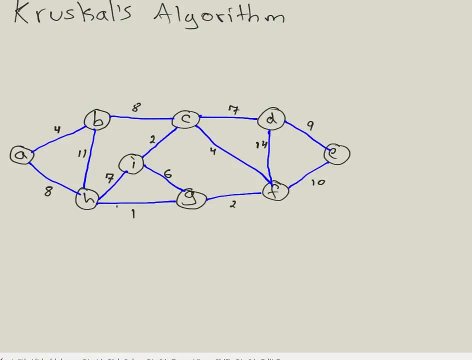 So we pick an edge- UV, in this case H and G- with the edge cost of 1.. Okay, we select this edge And we keep repeating this algorithm for this process until you reach all the vertices in the graph, And this will result in your minimum spanning tree. 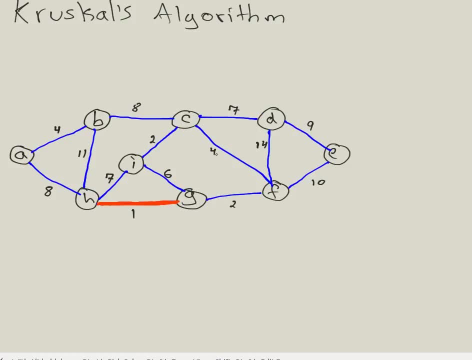 Okay, Next up. do we have any other ones in the graph? It doesn't look like it, So the next number up is 2.. In this case, we have two of them, And we can pick either one of them, because they will not form a cycle. 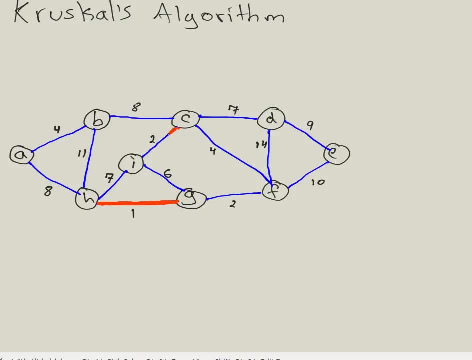 So let's go ahead and pick I and C, the edge between I and C, Okay. so that's in our tree, Okay, and we have another two here we can also pick, because it will not form a cycle. So let's go ahead and do that.